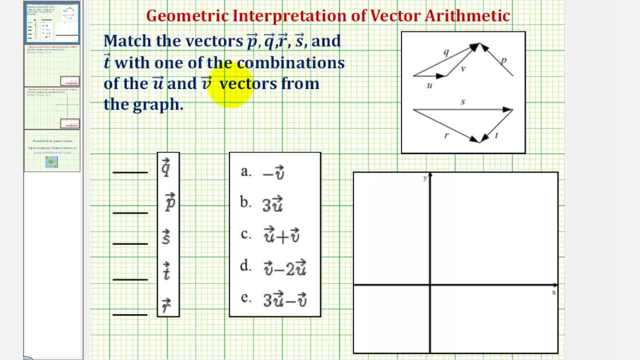 We want to match vectors P, Q, R, S and T, given here on the left, with one of the combinations of vector U and vector V from the graph. So we'll be matching A, B, C, D and E with these five vectors. Looking at the graph, notice how. here's vector U and. 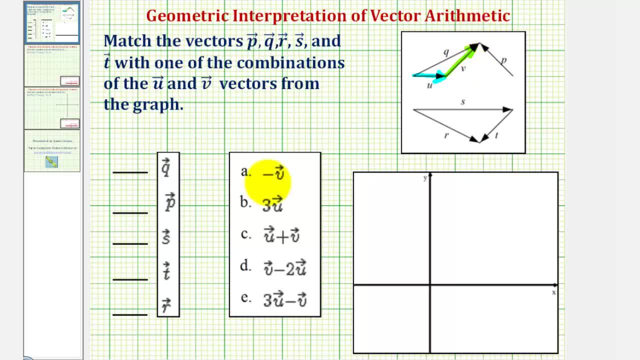 here's vector V. So, looking at A, we have the opposite of vector V or, if we want negative, one times vector V. So the opposite of vector V or if we want negative one times vector V, would be a vector that has the same magnitude or same length as. 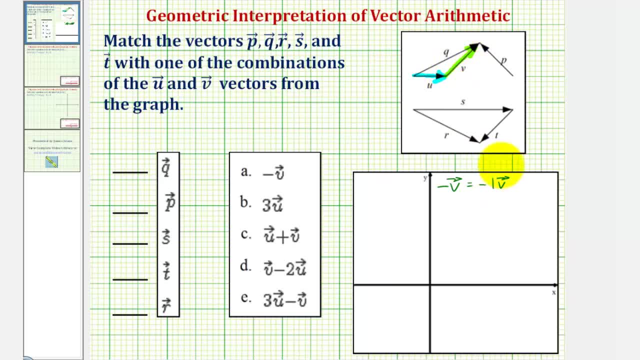 vector V, but in the opposite direction. So if we were to sketch vector V on the coordinate plane with the initial point at the origin, this would be vector V, and therefore the opposite of vector V, or negative one times vector V would be this vector, here in the opposite direction, with the same. 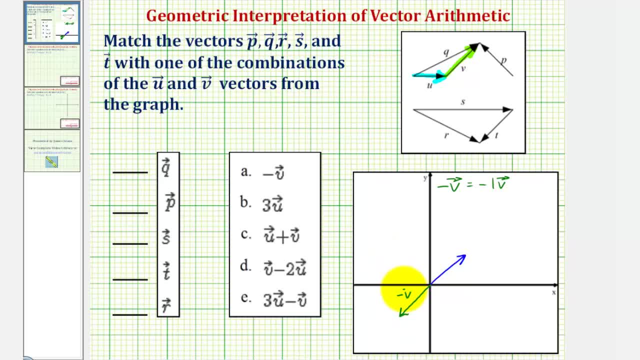 magnitude. So this is the opposite of vector V. So, looking at our graph, notice how this would match vector T. So A matches with vector T. Now notice for B. we have three times vector U. Well, if here's vector U three times vector U would be a vector in the same. 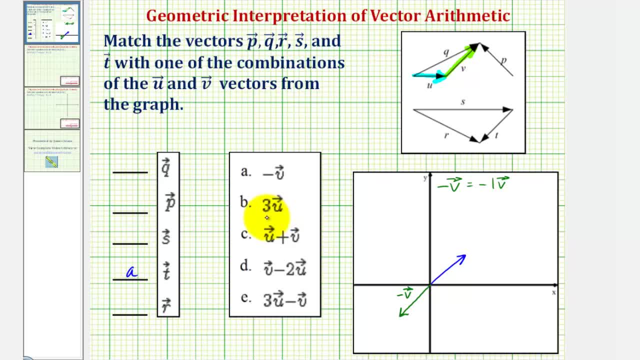 direction, but with three times the length of three times the magnitude. Looking at the graph, notice how we should recognize this. would be vector S, But if we did graph vector U on the coordinate plane with the initial point at the origin, it would look like this: 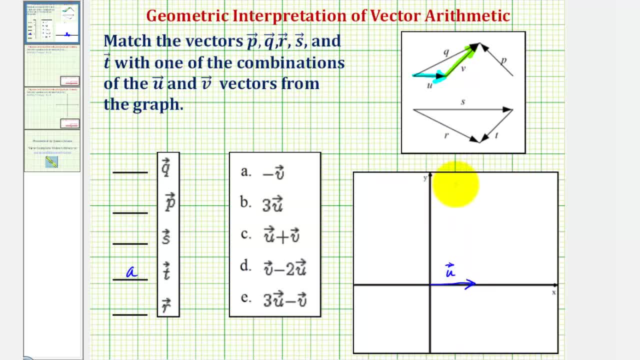 So this is vector U. So again, three times vector U would be a vector in the same direction with three times the magnitude, which would look like this: So the green vector here is three times vector U, which again matches vector S. So vector S would be B. Next we have vector U plus vector V. So 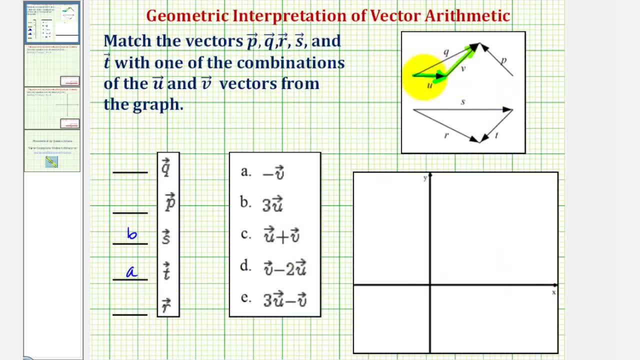 looking at the graph, notice how. here's vector U. If we place the initial point of vector V at the terminal point of vector U, as we see here, the resultant vector, or the sum, is the vector with the initial point at the initial point of vector U and terminal point at the terminal point of. 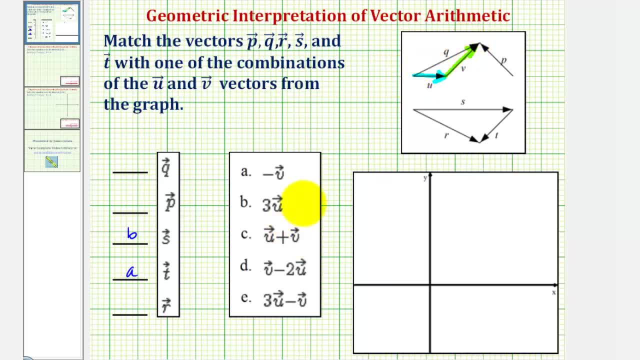 vector V, which is vector Q. So vector U plus vector V would be vector Q and therefore Q is C. And again, if we sketch this on the coordinate plane, we would first sketch vector U here, and then again we place the initial point of vector V at the terminal point. 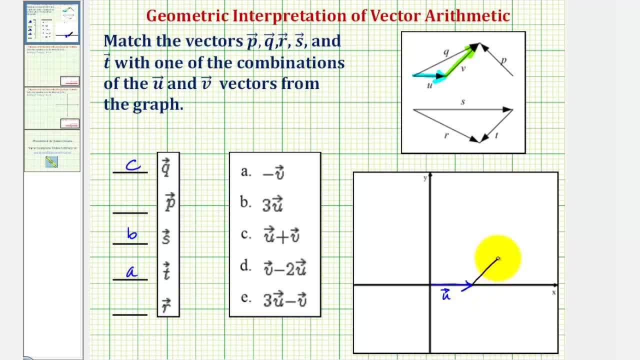 of vector U, which would look like this, And the resultant vector, or the sum, would be this vector, here The vector with the initial point at the initial point of vector U and the terminal point at the terminal point of vector V. 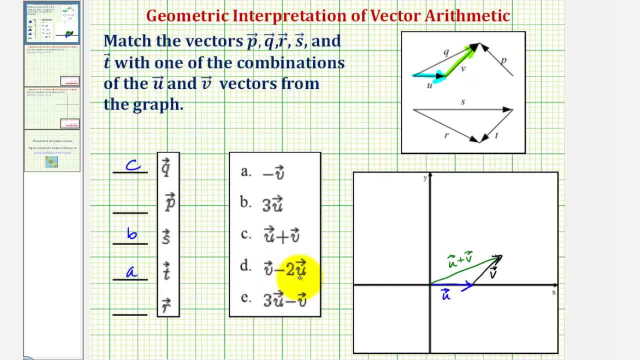 Now for D. we have vector v minus two times vector u, So, if it's helpful, we can write vector v minus two times vector u as vector v plus negative two times vector u. This one's not shown in our graph, so let's go ahead and sketch this on the coordinate plane. 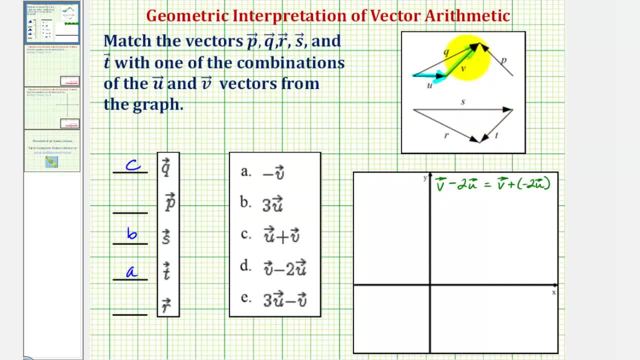 We'll begin by sketching vector v with the initial point at the origin, which would look like this: And now we'll add negative two times vector u. Well, negative two times vector u would be the vector that has twice the length or twice the magnitude. 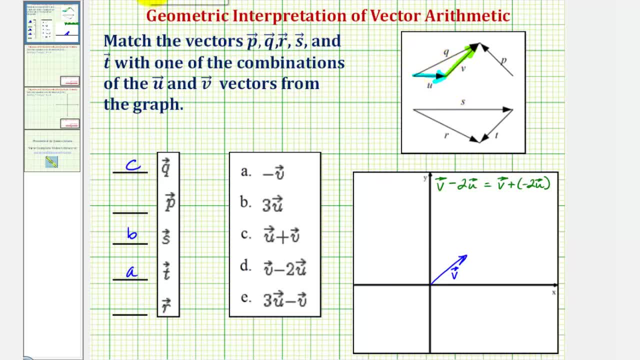 of vector u, but in the opposite direction, which would look like this: So this would be negative two times vector u. So the resultant vector is the vector with the initial point, which would be the initial point of vector v, and the terminal point of negative two times vector u. 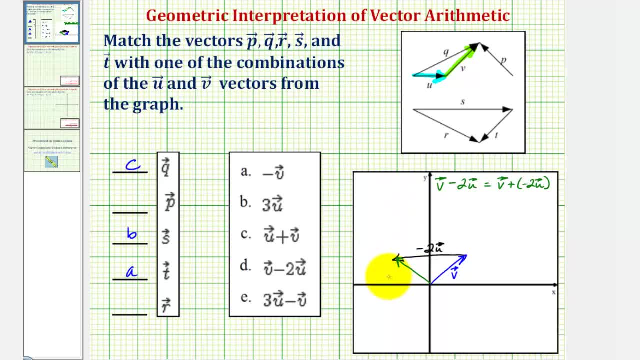 or this vector here. So again, this is v minus two times u. Looking at our graph, notice how this vector here resembles or matches vector p. So vector p would be d and then finally we have e, 2001.2, 3 times vector p.